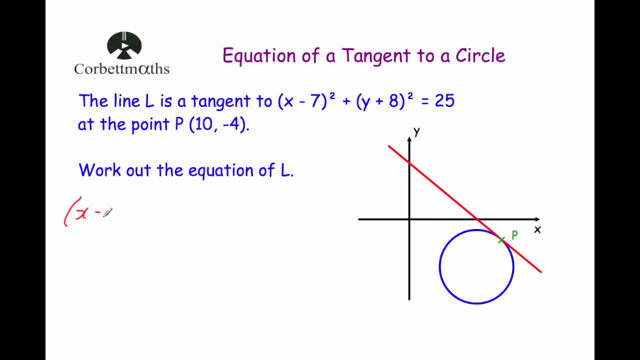 of the circle. So the equation of a circle is in the format: x minus a plus y minus b equals r squared. So the centre of the circle is the point a- b. So if we look at the equation of the circle we've been given, we know that a is going to be equal to 7. So the centre, 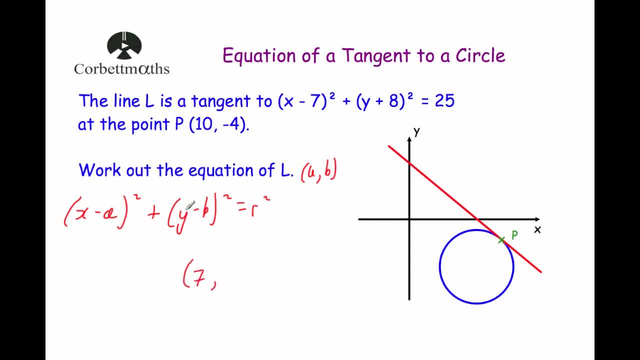 of the circle will be 7.. And then, looking at the y-coordinate, well, it's y minus b, but this is plus 8, so the centre of the circle would be the point 7 minus 8.. So the centre of the circle C is the point 7 minus 8.. Now we know the centre of the circle and we know 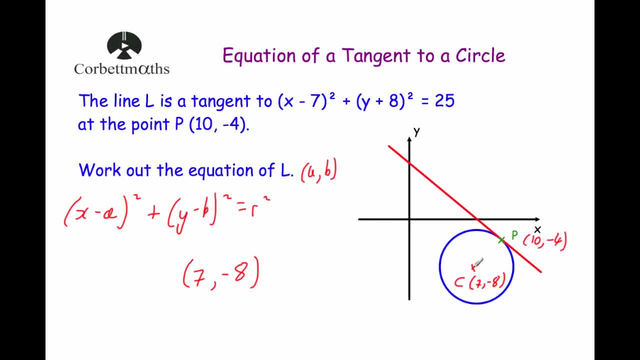 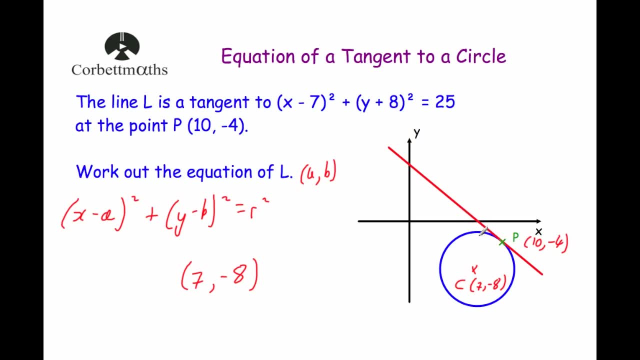 what the point P is, which is 10 minus 4, we can work out the gradient of the line joining those, the gradient of the radius, and then, once we know the gradient of the radius, we can work out the gradient of the tangent by just working out the negative reciprocal. 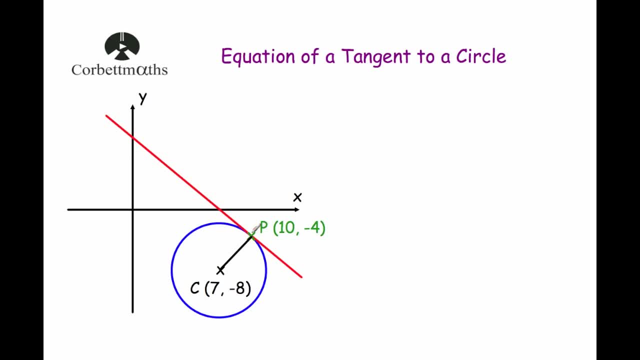 because these are perpendicular lines. Okay, so let's work out the gradient of the radius. So let's call the points x1, y1, and x2, y2. So the gradient M is equal to y2 minus y1 over x2 minus x1. So let's substitute in those values so M equals y of 2, that's going. 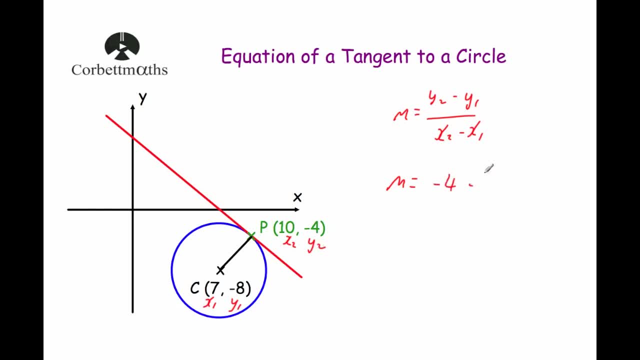 to be minus 4, minus y1, so it's going to be minus minus 8, over x2, that's 10, minus x1, that's 7.. So that's going to give us minus 4, minus minus 8, so it's going to be minus. 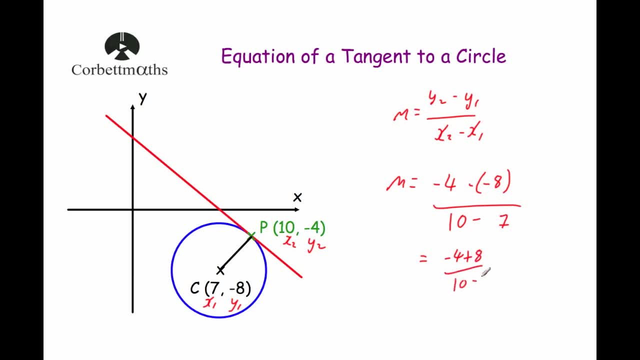 4 plus 8.. Over 10 minus 7, that's going to be minus 4 plus 8, that's 4 over 3.. So the gradient of this line, CP, will be equal to 4 thirds. So that means the gradient of the tangent. 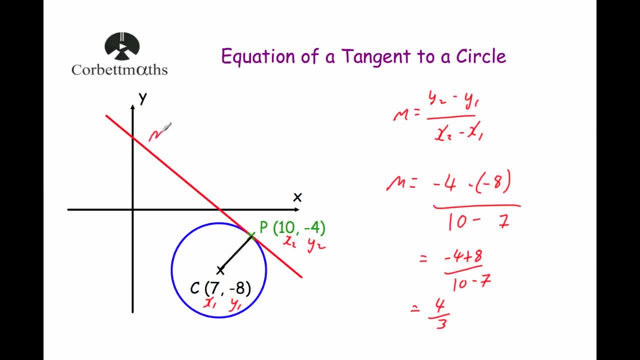 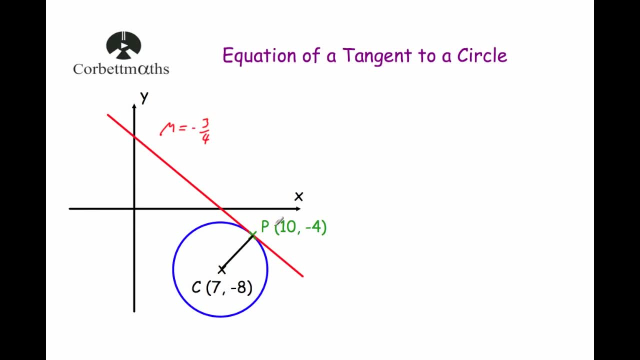 will be the negative reciprocal of that. So that means the gradient of the tangent L1 is equal to minus 3 quarters. So now that we know the gradient of the tangent is equal to minus 3 quarters and the tangent passes through the point 10 minus 4, we can work. 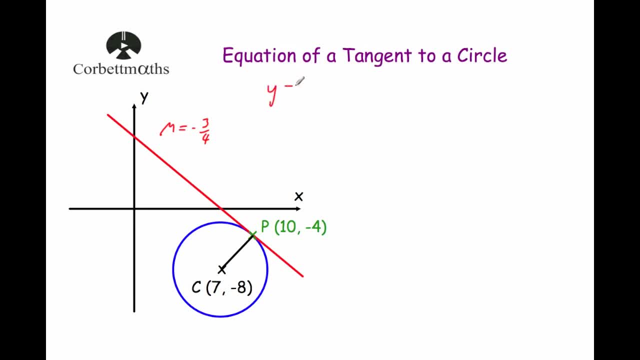 out the equation of that tangent. Now we could use the equation y minus y1 equals M, bracket x minus x2.. Or alternatively, we could just use y equals M, x plus c and substitute in our values And that's the version I'm going to use. So for our coordinate it has an x coordinate of 10.